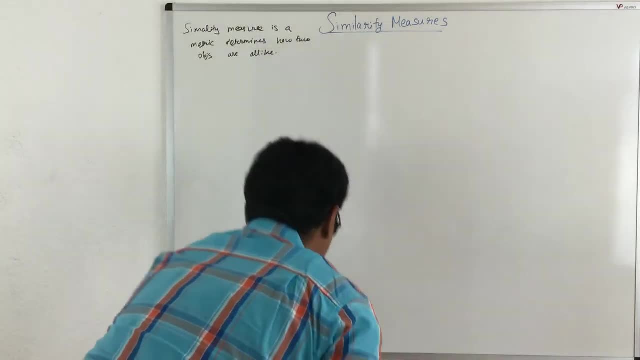 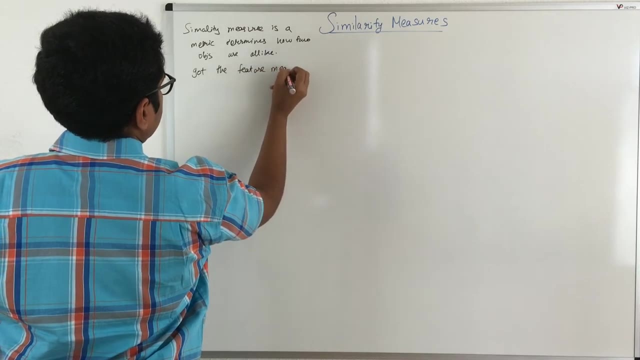 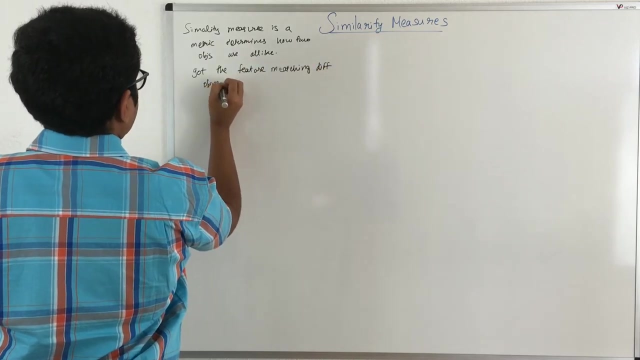 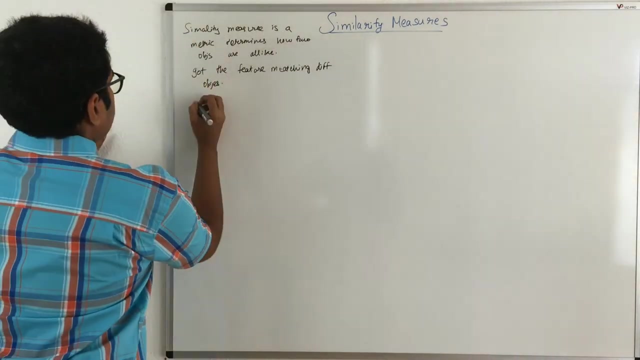 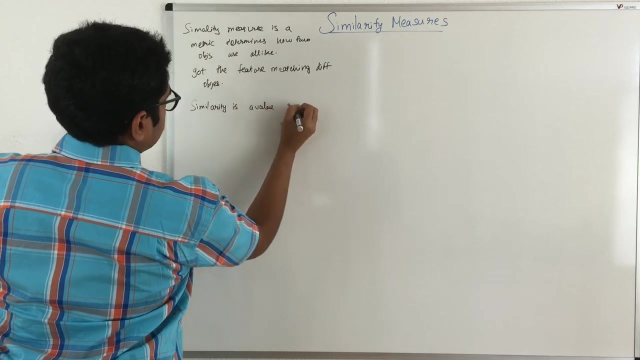 So essentially, what I have did is I've just got the features, or the feature matching between different objects. So, based upon various dimension, we just categorize two different objects: How similar are they? So the similarity measure is a value which ranges from 0 to 1.. 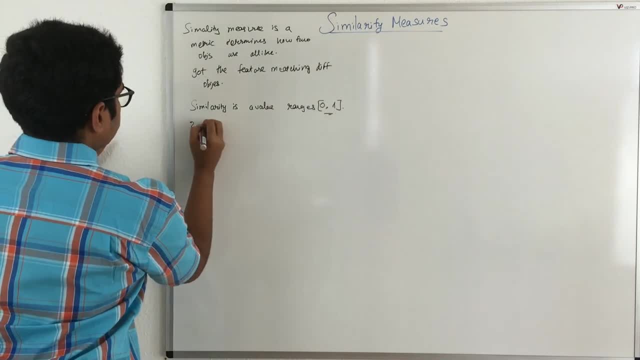 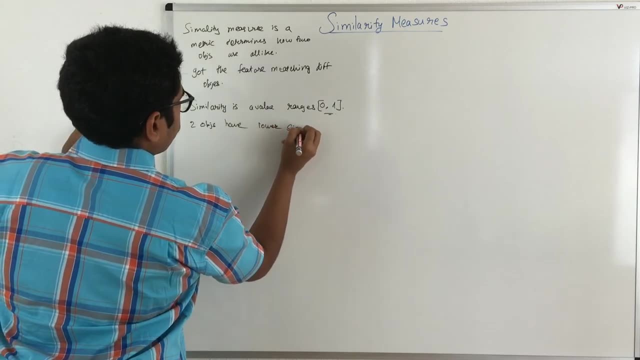 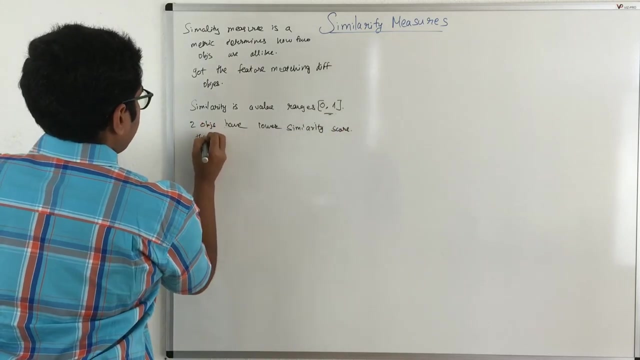 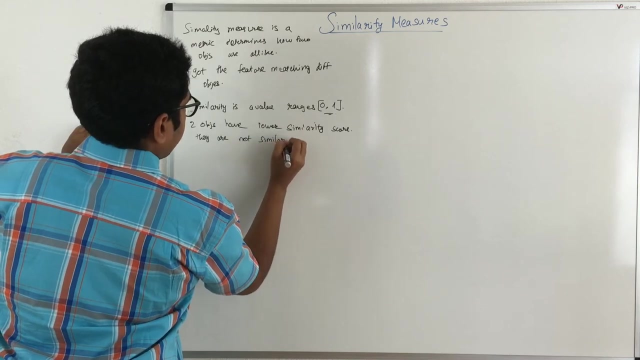 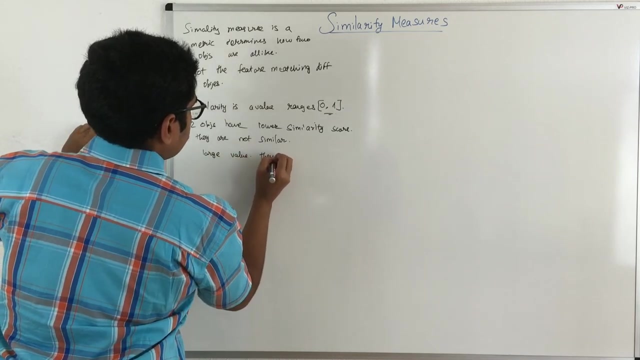 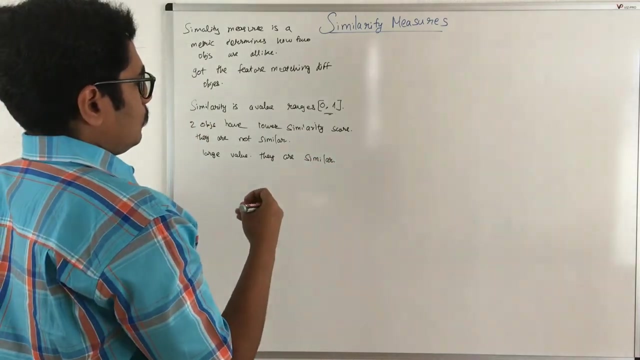 So it is in this range. So if two objects Have lower similarity score or the distance is very small, That means they are not similar, or if they have larger value of similarity, Then they are. similar Means how closely two objects are there, or what is the characteristic that distinguishes between one object. 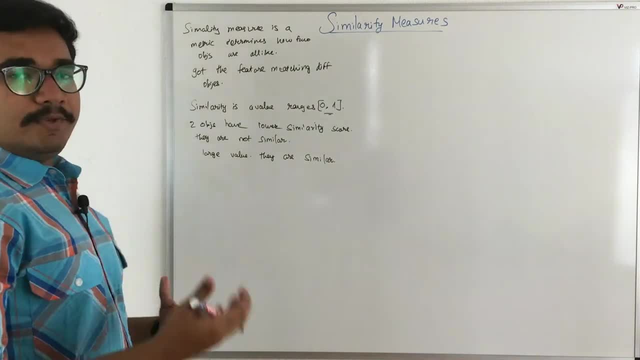 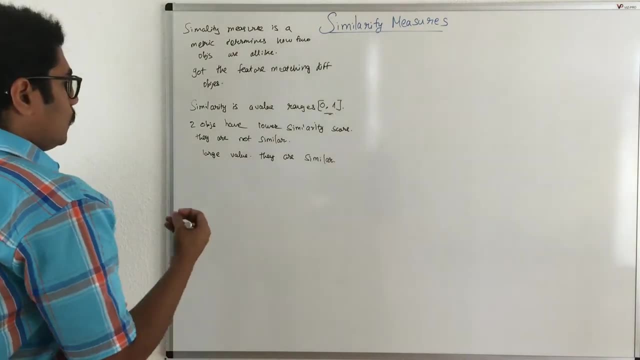 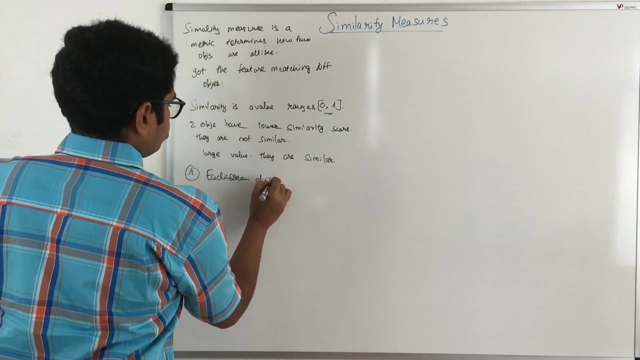 and the other object. now there are certain ways where we estimate, or certain mathematical measures where we estimate the similarity measures in clustering. So I'll give a overview of those. So very first is we have the Euclidean distance. So say, for example: 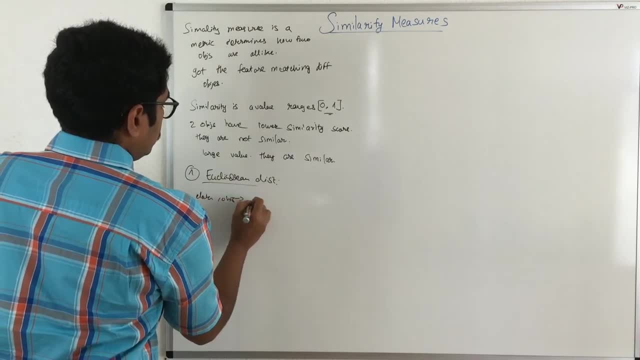 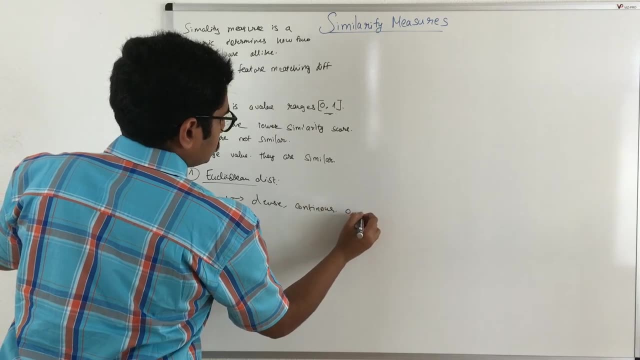 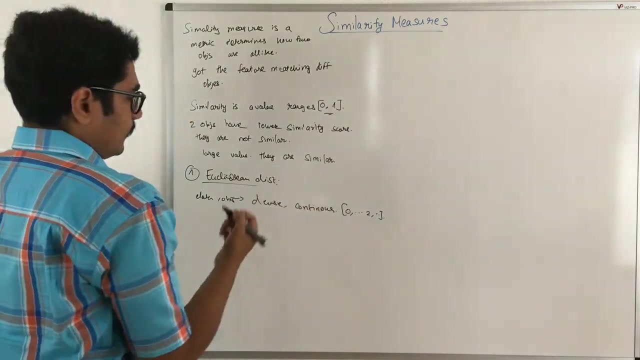 our data sets or objects are very dense means in large number or they are continuous. Like you have value ranges 0, 1, 2, 3, up till some number or some decimal point, So we mainly use Euclidean distance when we have dense or continuous attributes. 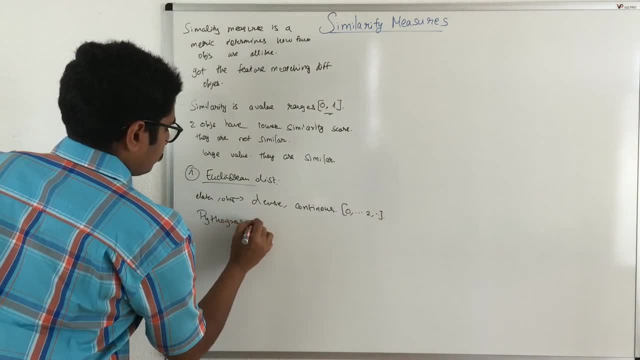 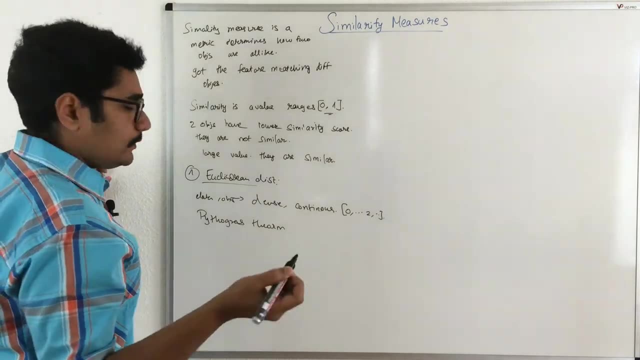 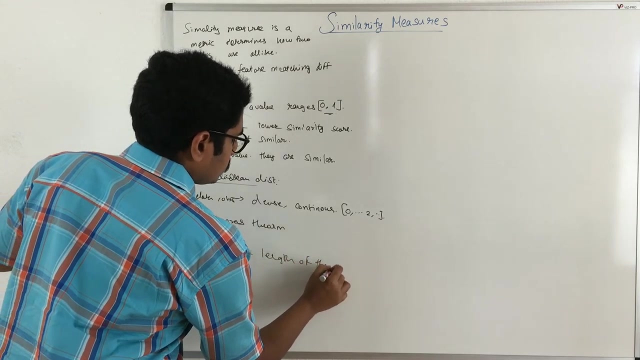 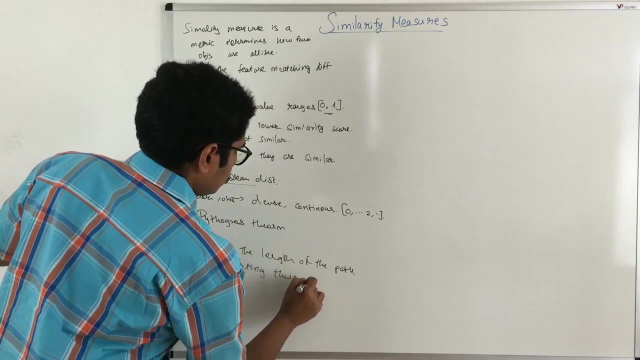 So we mainly use Pythagoras theorem or Pythagoras formula in order to calculate the distance between two objects. So Euclidean distance between any two points. say we have X and Y- is the length of the path Connecting these objects. Say for instance: 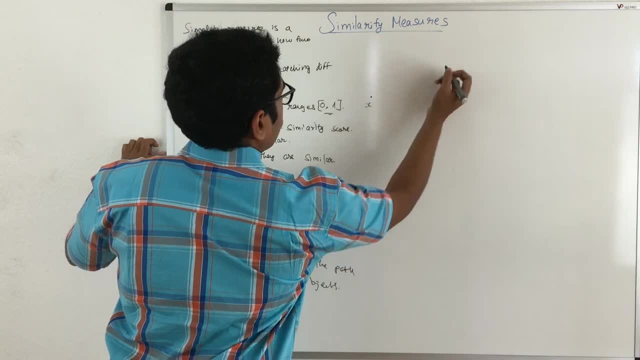 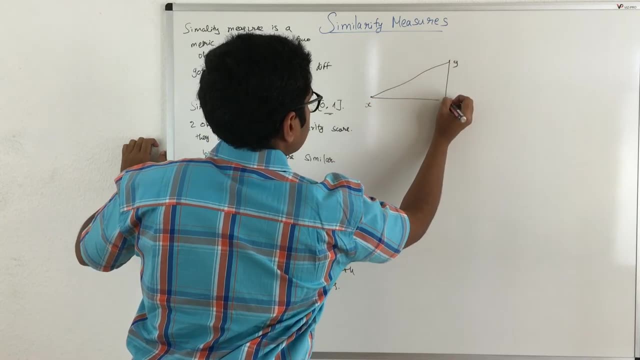 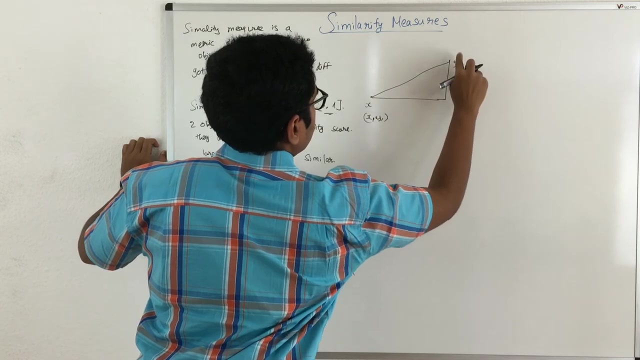 I have this point: say this is X and this is Y, now This is the length that connects these two. say this has coordinates X 1 and Y 1 and this has X 2, Y 2. just consider this as B and this as A. 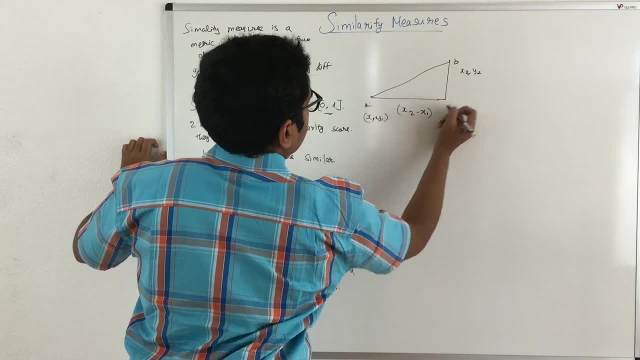 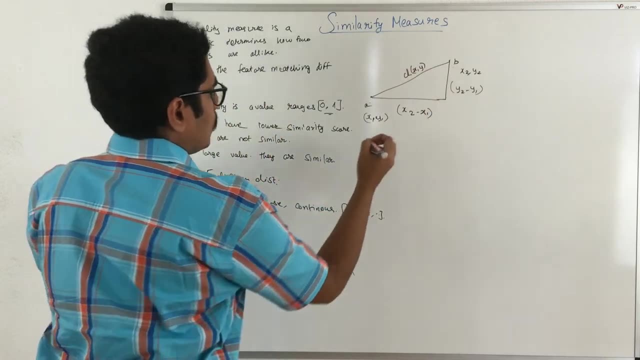 So what? this horizontal distance is X 2 minus X 1, and this will be Y 2 minus Y 1.. So this distance is the Euclidean distance. So how you estimate mathematically? so distance between two points is given as square root of summation. 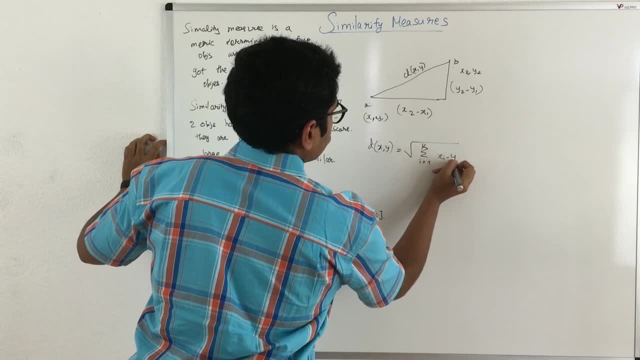 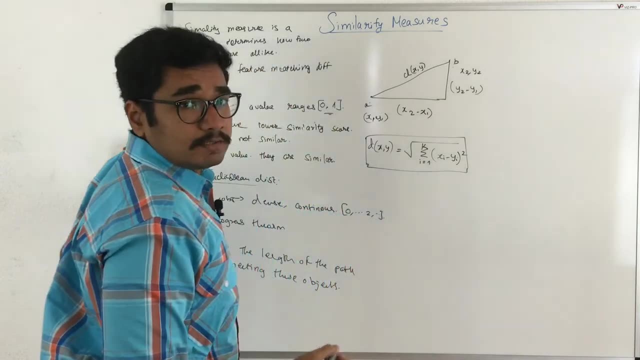 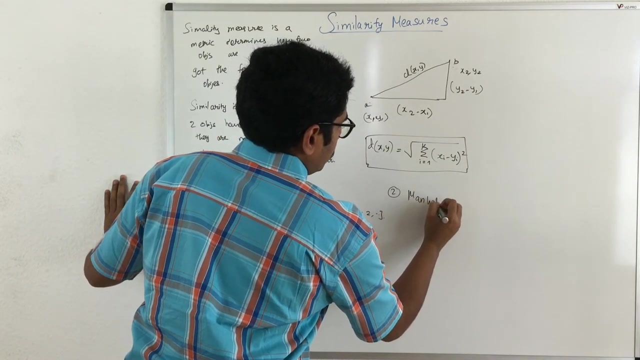 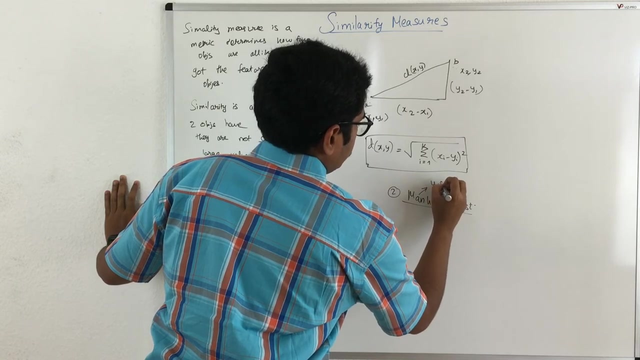 I runs from 1 to K, X I minus Y I the whole square. So this is how you calculate Euclidean distance with the help of Pythagoras theorem. Now, secondly, we have distance called as Manhattan distance, So this name is place or a city in US called as Manhattan. 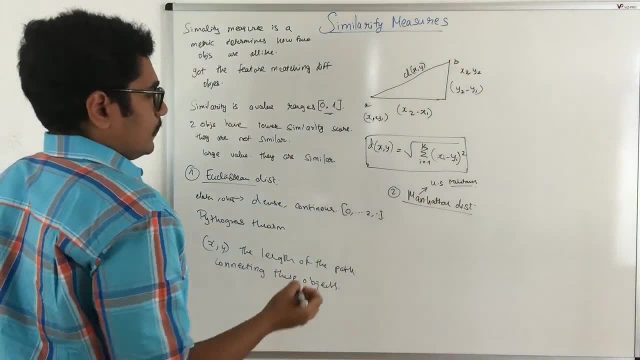 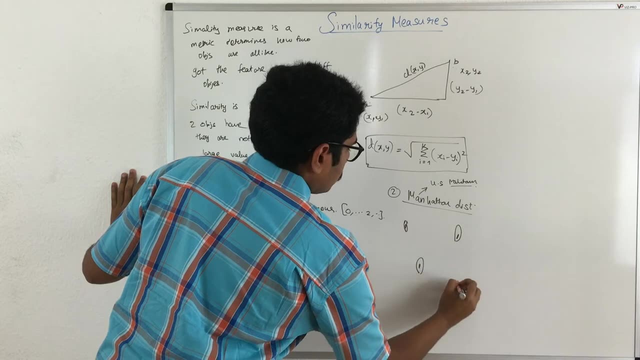 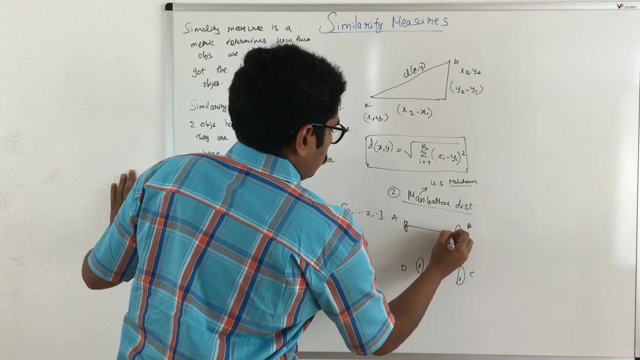 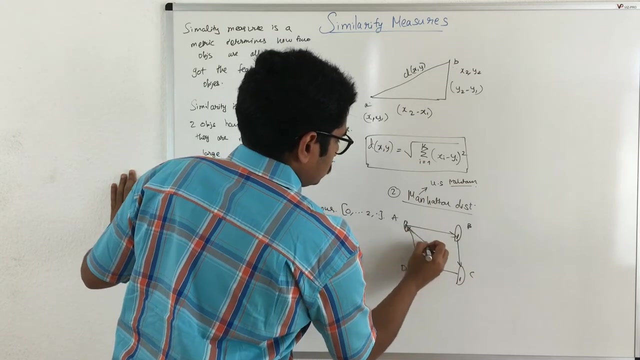 So from there we got actually this name: Manhattan distance. So say, for example, we have two locations, say two points, This is one location, These are four different locations, say A, B, C, D. So if you want to find the distance from this point to this point, or this point to this point, or inter city distances connecting between these two points internally, 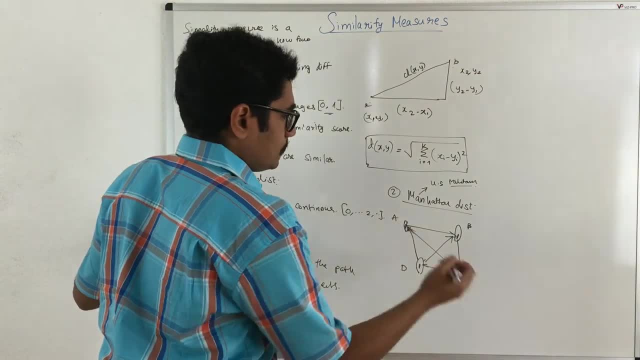 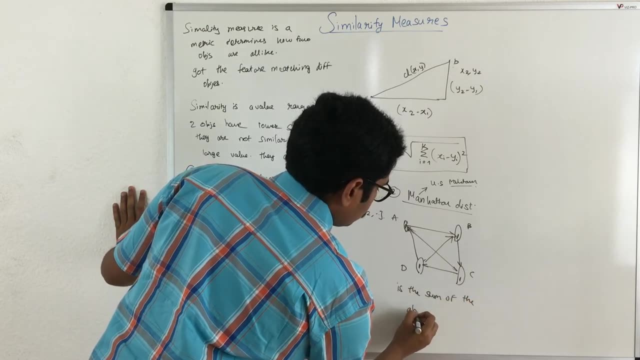 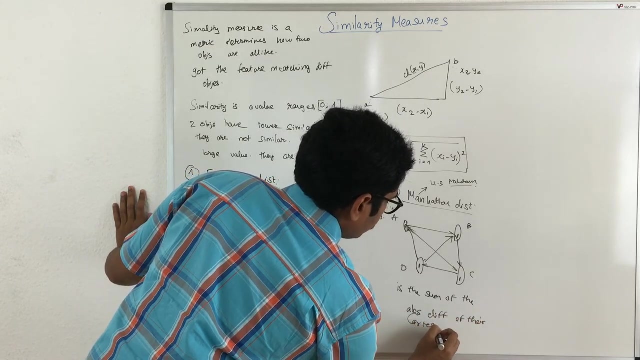 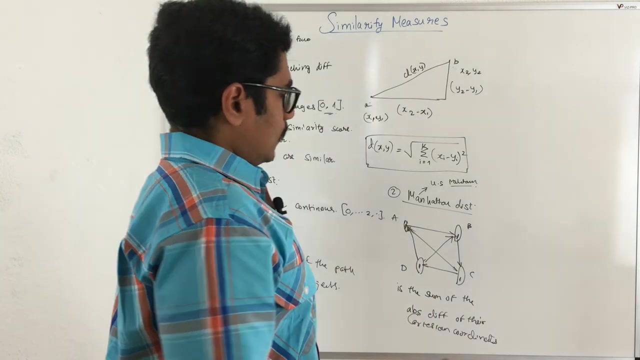 so we mainly use Manhattan distance in this. So Manhattan distance between any two points is the sum Of the absolute difference of their Cartesian coordinates. What this means is basically: in graph or in geometry you have different planes, So you calculate the longitude, latitude. 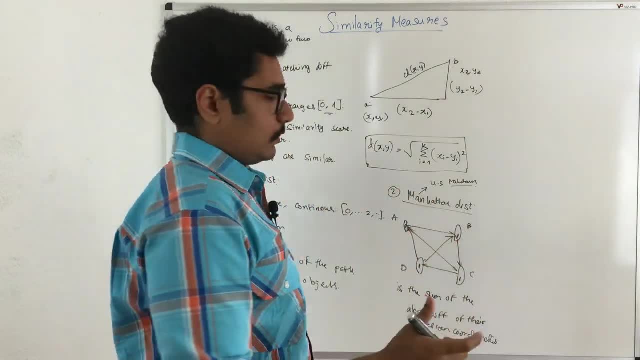 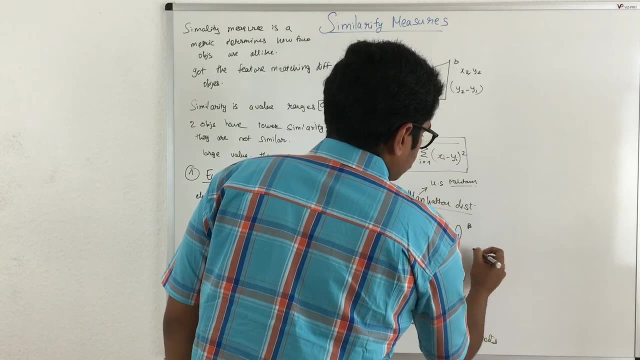 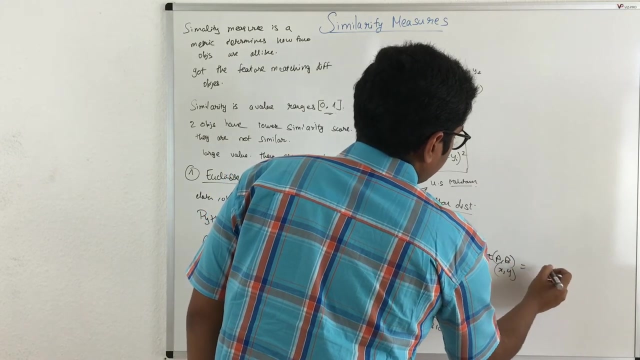 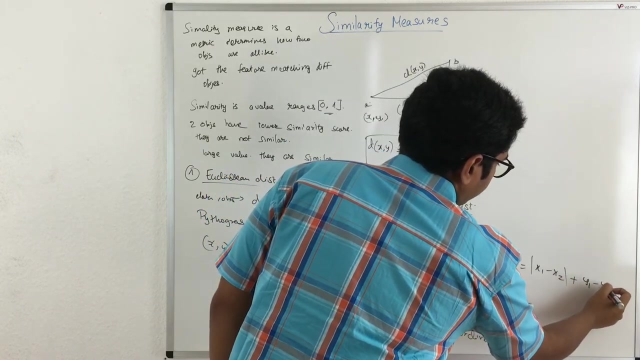 So you have different coordinates. So there you Mainly use Manhattan distance in order to calculate the separation of two different points or two different objects. So mathematically it is given has. so distance between any two points, A or B, or say X or Y, is given as X 1 minus X 2, the absolute difference of their coordinates. 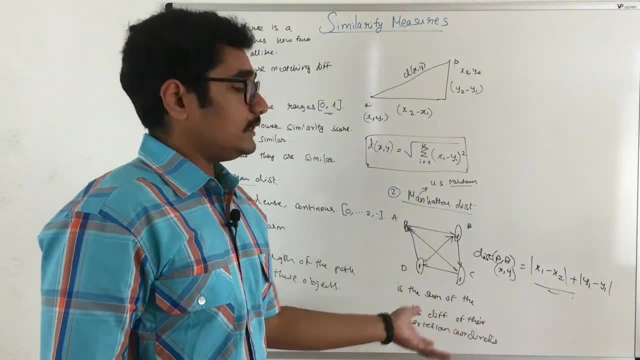 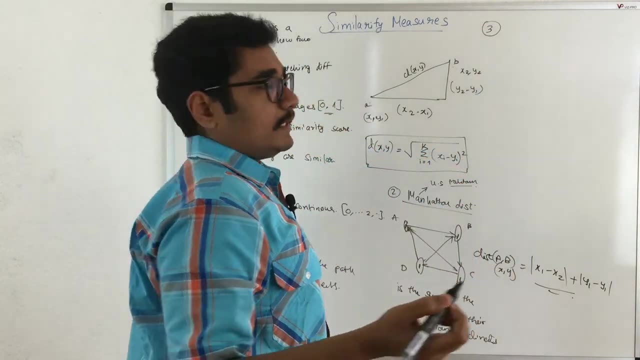 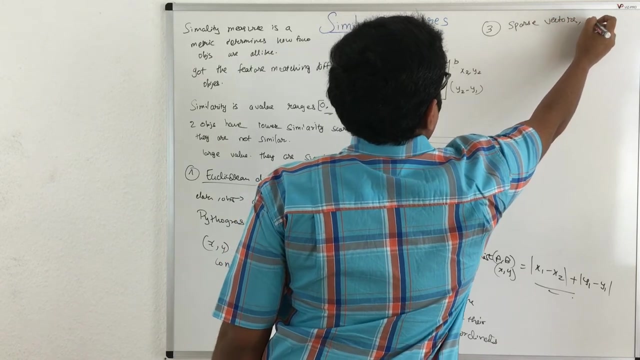 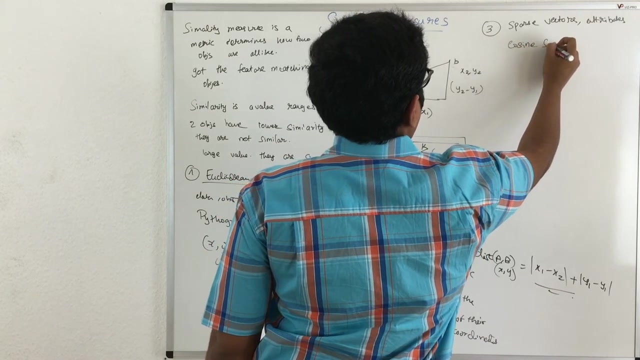 and you submit up. So this is how you give the Manhattan distance between any two points or any two locations. Now, third type is when we have sparse data, means we have very few data, or in fact we can say sparse vectors or attributes. There we mainly use cosine similarity. 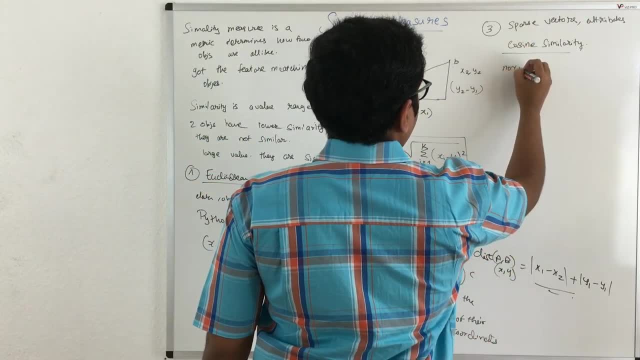 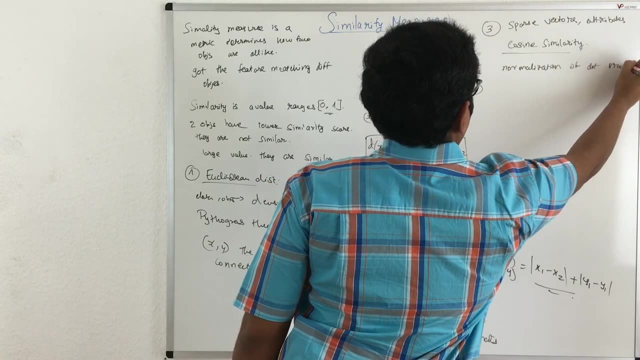 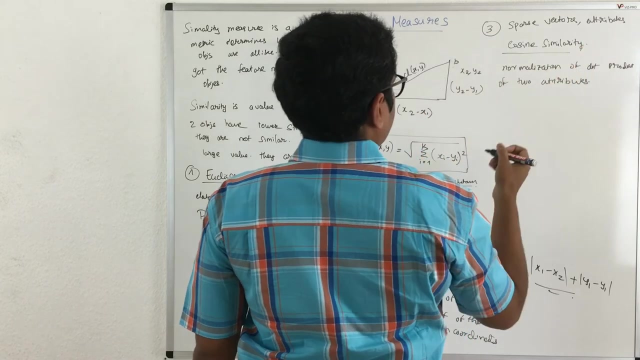 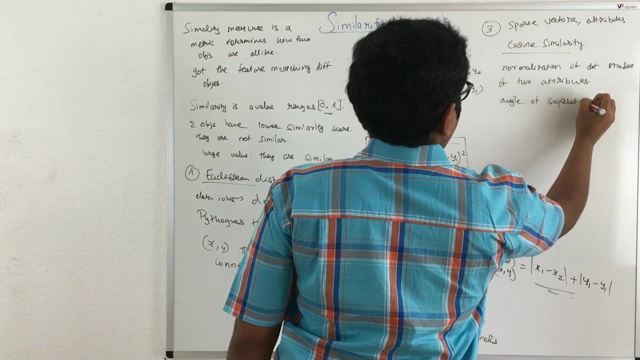 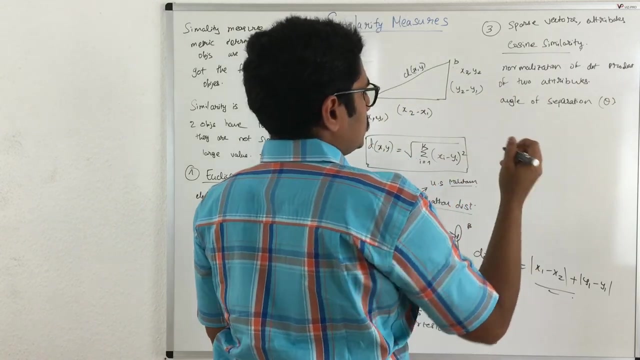 So cosine similarity essentially finds normalization Of the dot product Of two attributes. So it basically finds the angle of separation. We can call it as theta here, and so cosine similarity or cosine distance is mainly used, or it judges the orientation Of two input vectors. 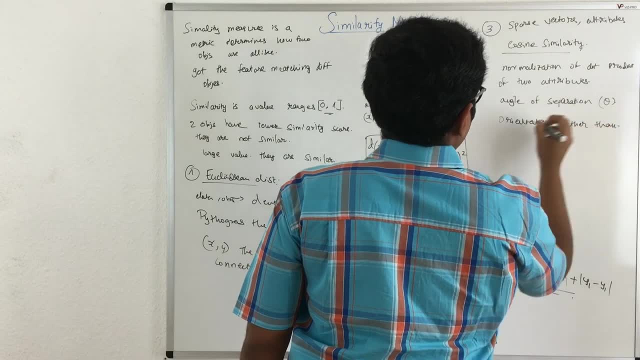 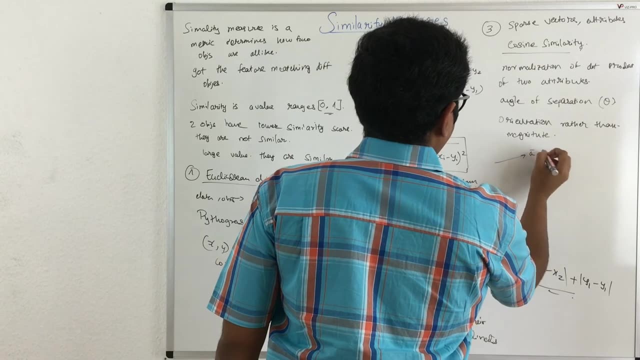 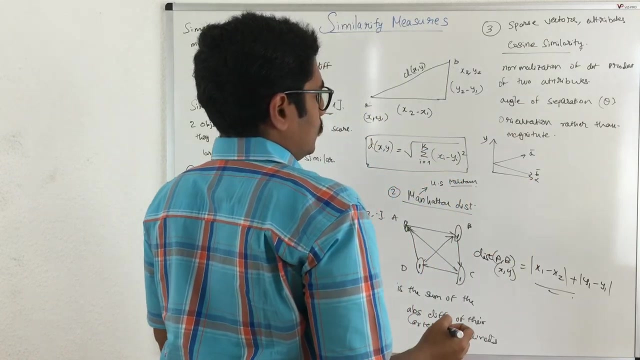 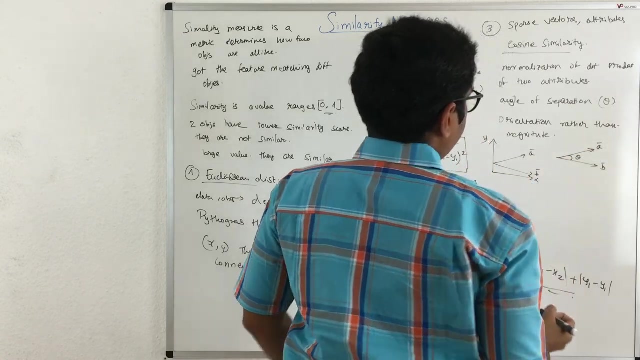 Rather than Their magnitude. Say, you have two input vectors like this, A and B, over two planes, You have Y and X. So how you estimate if there are Two input vectors, A and B, and there is a value theta, So how you estimate this theta value? 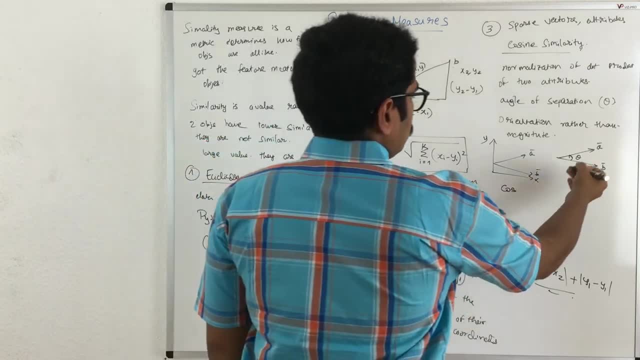 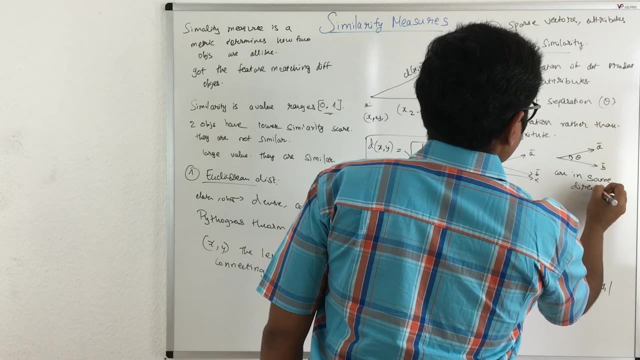 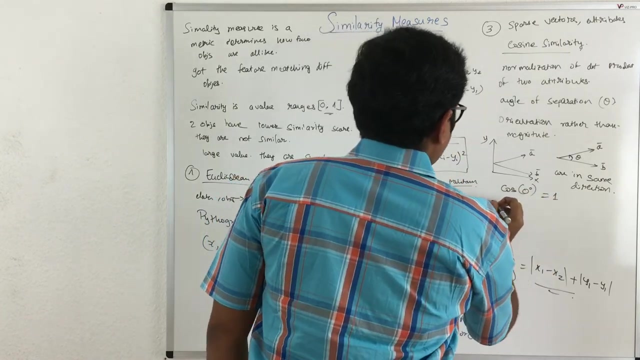 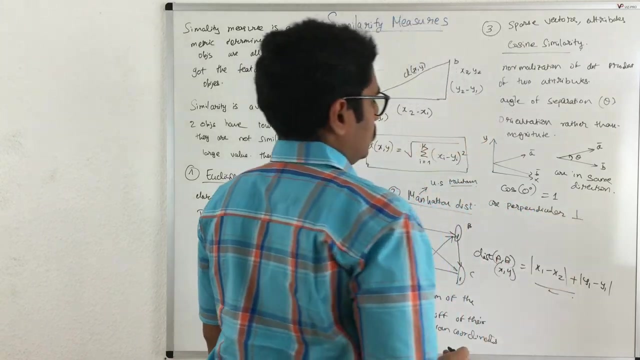 Is basically by taking their cosine value. So if the two input vectors are in same direction, What you take is cosine of 0 degree, that is one. if they are perpendicular to each other. That is like this. So you have the cosine degree of 90, that is 0.. 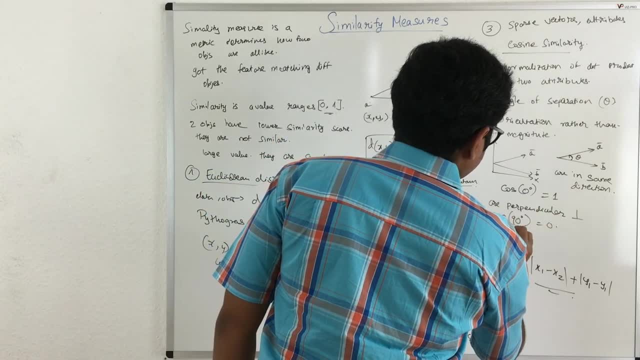 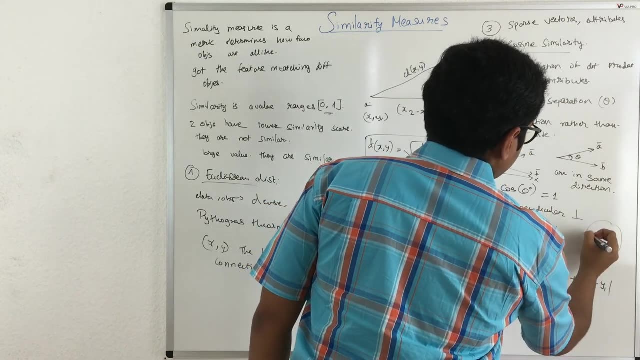 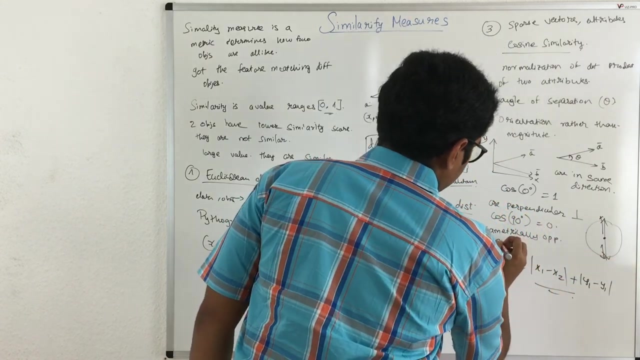 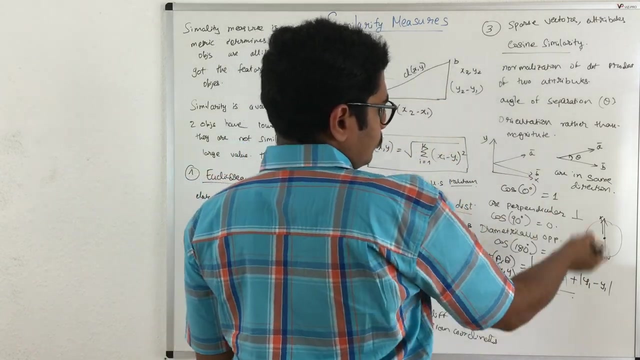 Else they are diametrically opposite. Something like you have a circle like this: So if they are here, one is towards this direction and there is towards this direction. So it's separated with 180 degree, So it is negative 1, and so you have different values.